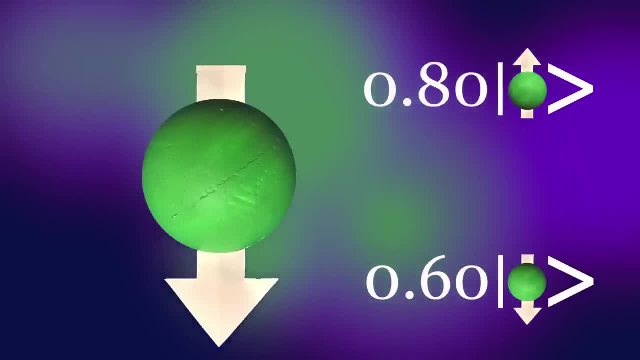 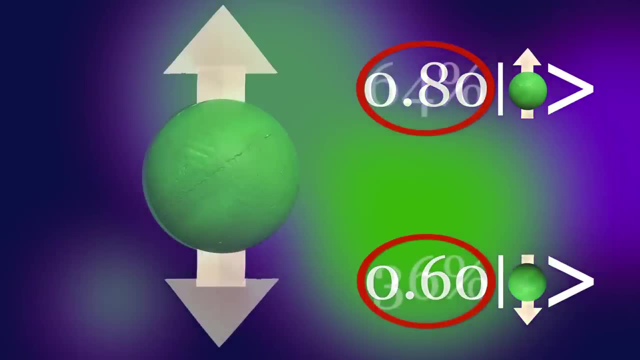 Now, when you measure the spin, it will be either up or down, But before you measure it, the electron can exist in what's called a quantum superposition, where these coefficients indicate the relative probability of finding the electron in one state or the other. 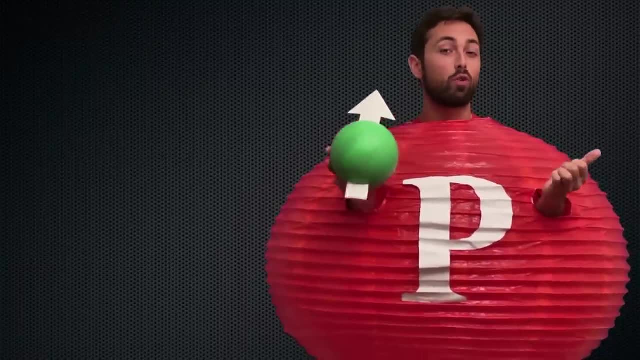 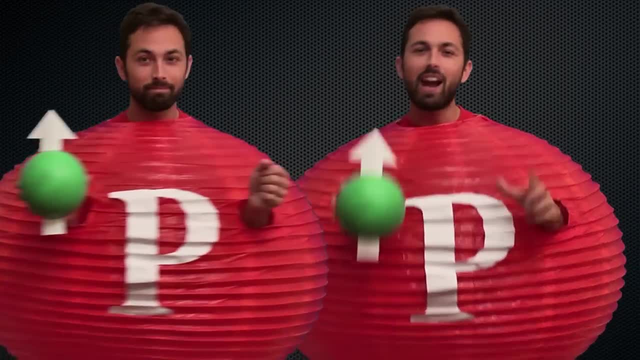 So let's take a look at one of these. So let's take a look at one of these. So let's take a look at one of these. Hello, hi. Now there are four possible states of these two electrons. 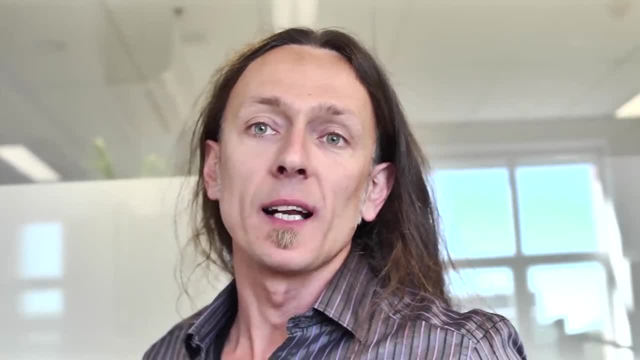 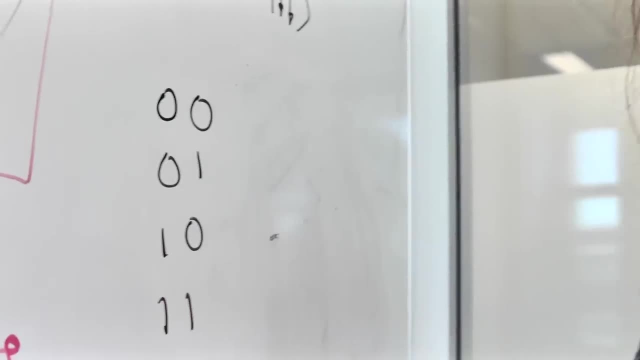 You could think that, well, that's just like two bits of a classical computer, right? If you have two bits, you can write 00,, 01,, 10,, 11,. right, It's four numbers. But these are still just two bits of information, right? 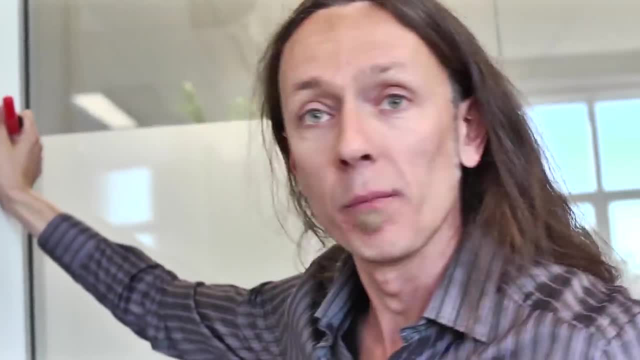 All I need to say to determine which one of the four numbers you have in your groundwater are quote–unquote zero and zero nine, Hi, Hello, раз Now. I'm terrible at this. I need an answer Now. I'm lost in this war. I'm just thinking too. Here's a new hint. 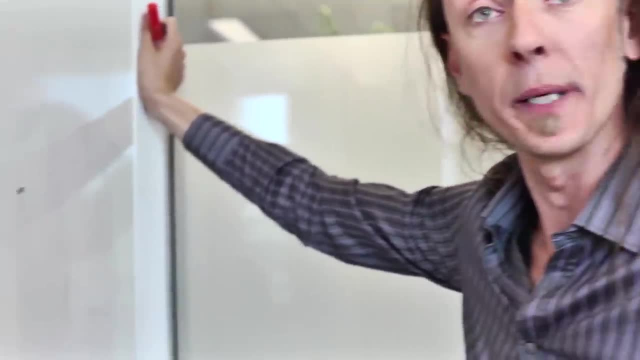 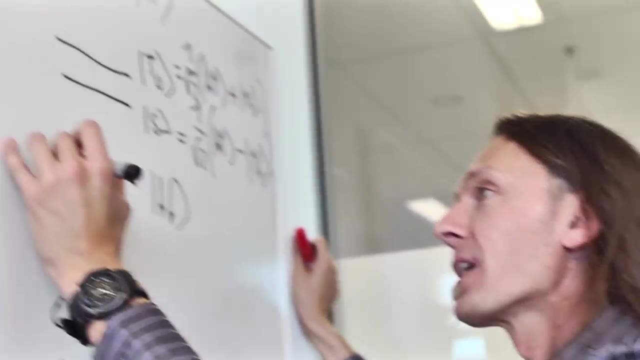 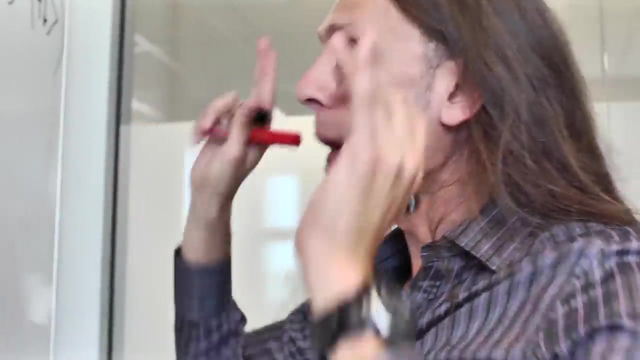 computer code is the value of the first bit and the value of the second bit. Here instead, quantum mechanics allows me to make superposition of each one of these four states, So I can write a quantum mechanical state which is perfectly legitimate. that is some. 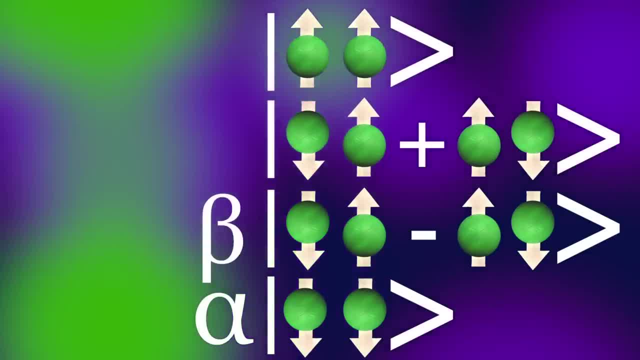 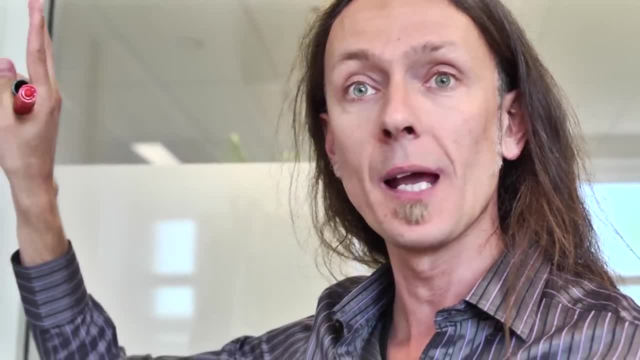 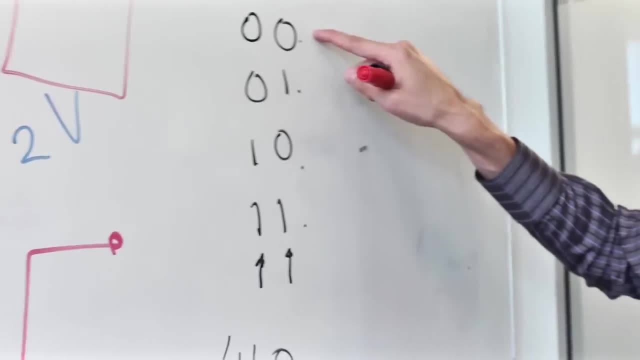 coefficient times this plus some coefficient times that plus some coefficient times that plus some coefficient. So to determine the state of this two-spin system, I need to give you four numbers, four coefficients, Whereas in the classical example of the two bits, I only need to give you two bits. 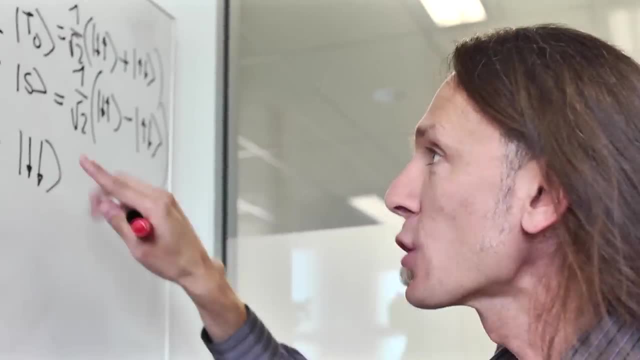 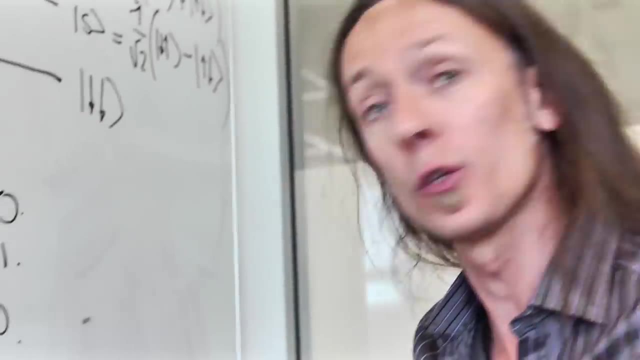 So this is how you understand why two qubits actually contain four bits of information. I need to give you four numbers to tell you the state of this system, whereas here I only need two. Now, if we make three spins, we would have eight different states. 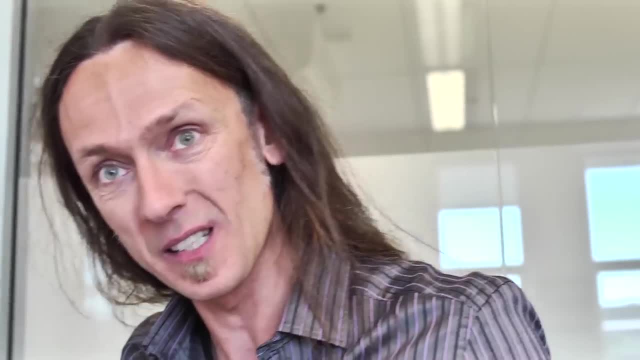 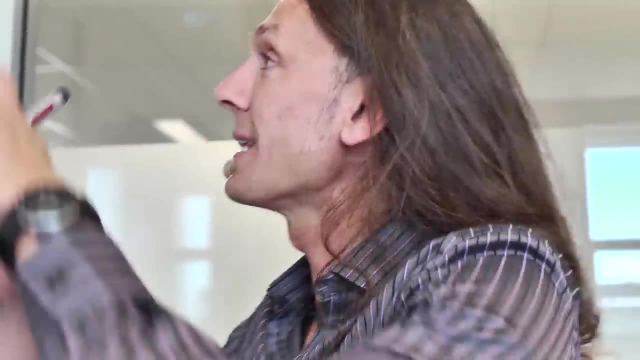 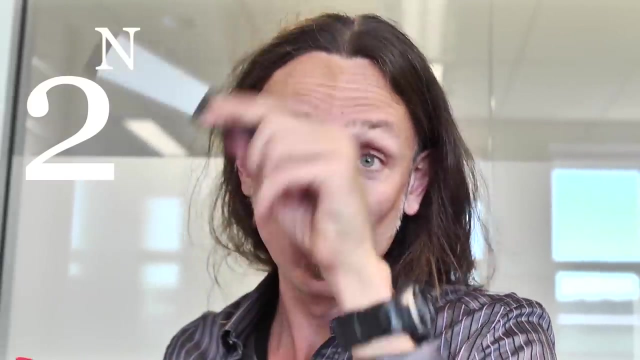 I need two. I need to give you eight different numbers to define the state of those three spins, whereas classical is just three bits. If you keep going, what you'll find is that the amount of equivalent classical information contained by n qubits is two to the power n classical bits. 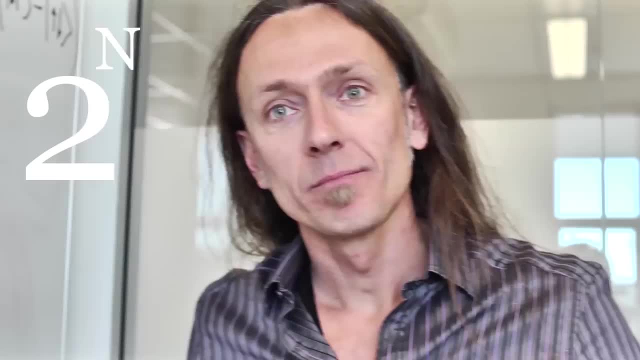 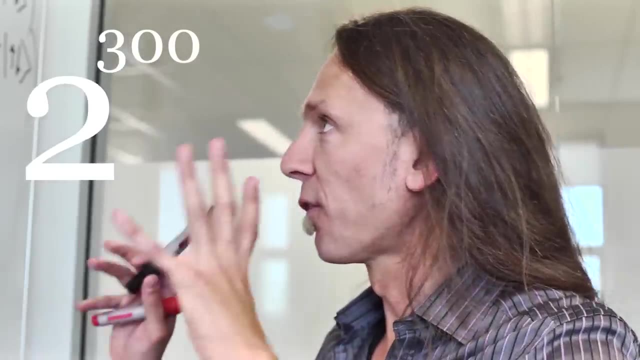 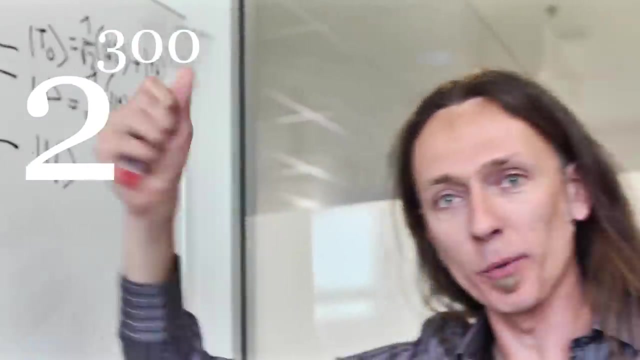 And, of course, the power of exponentials tells you that once you have, let's say, three hundred of those qubits in what we call the fully entangled state, so you must be able to create these really crazy states where there is a superposition of all three hundreds being. 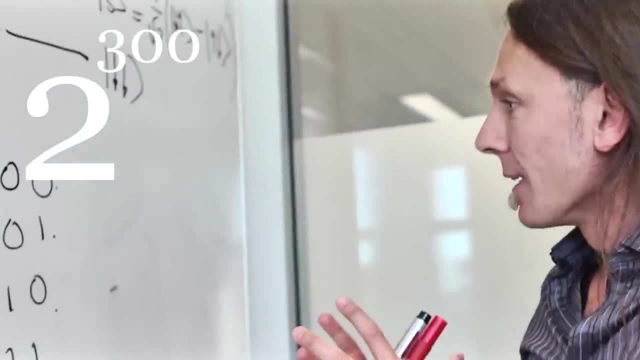 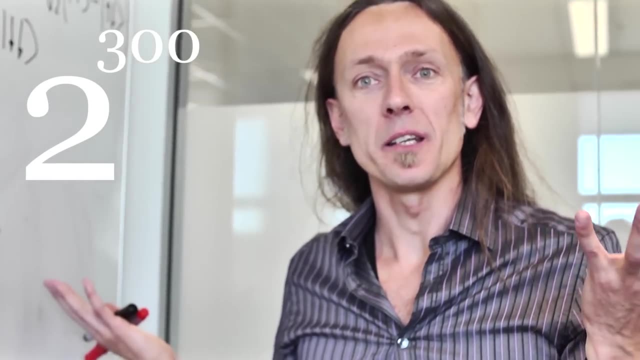 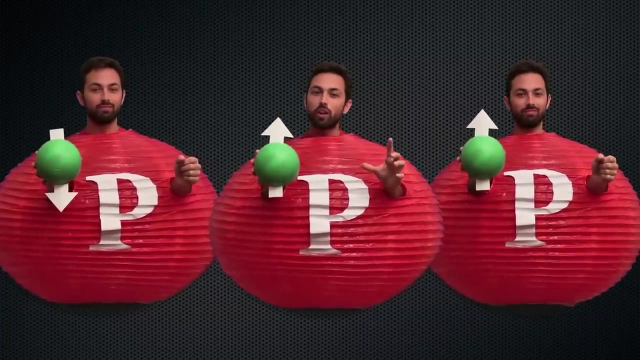 one way, and another way, and another way and so on. then you have like two to the three hundred classical bits, which is as many particles as there are in the universe. But there's a catch: Although the qubits can exist in any combination of states, when they are measured they must fall into one of the basis states and all the other information about the state before the measurement is lost. So you don't want generally to have as the final result of your quantum computation something that is a very complicated superposition of states, because you cannot measure a superposition. 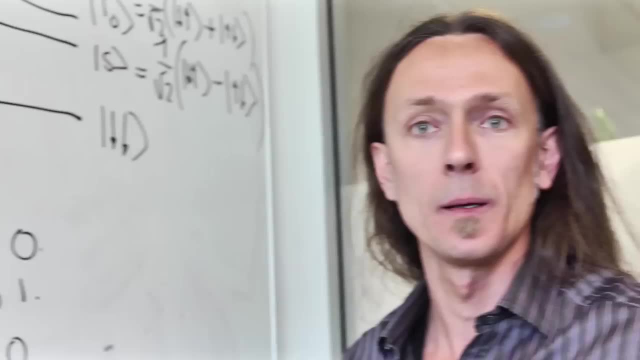 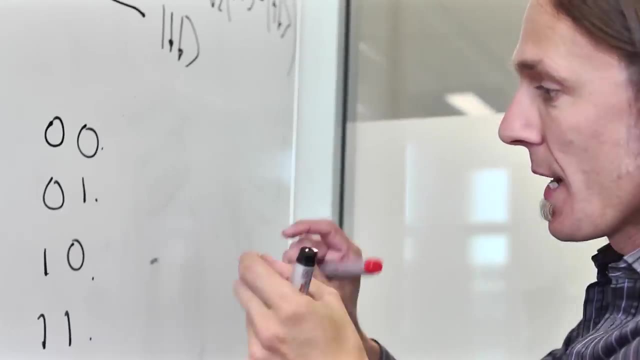 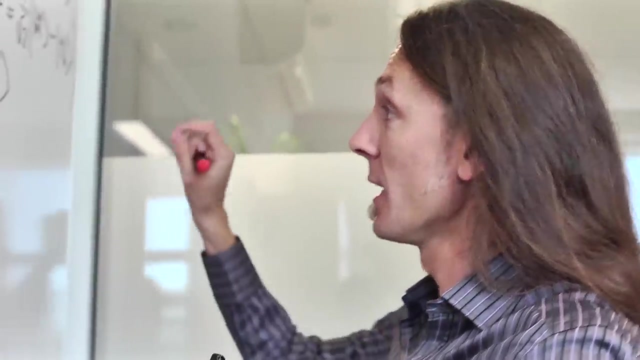 You can only measure one of these basis states, Right Like down, down, up, up, Yeah. So what you want is to design the logic, The logic operations that you need to get to the final computational result, in such a way that the final result is something you're able to measure. 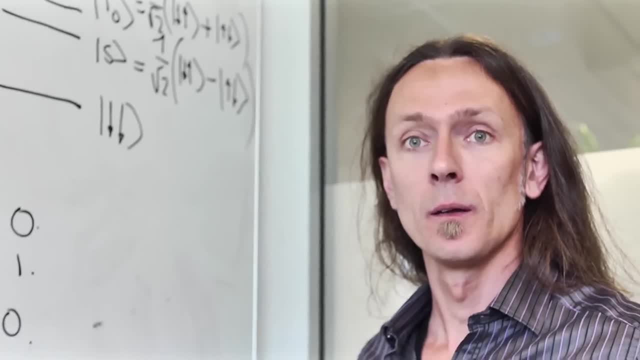 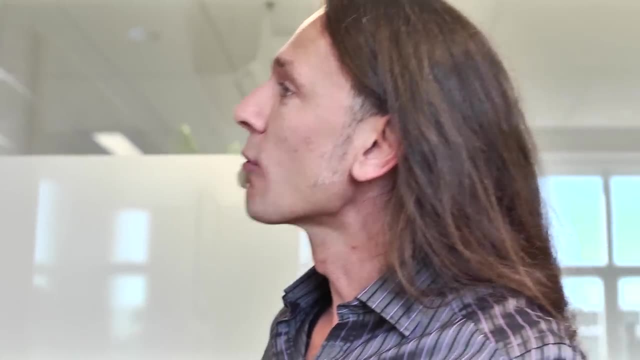 It's just a unique state. essentially, That's not trivial. That's not trivial And it's essentially- I'm kind of stretching things here, but I guess it's to some degree the reason why quantum computers are not a replacement for classical computers. They're not. No, they're not. They're not universally fast, They're only. They're only faster for special types of calculations, where you can use the fact that you have all these quantum superpositions available to you at the same time to do some. 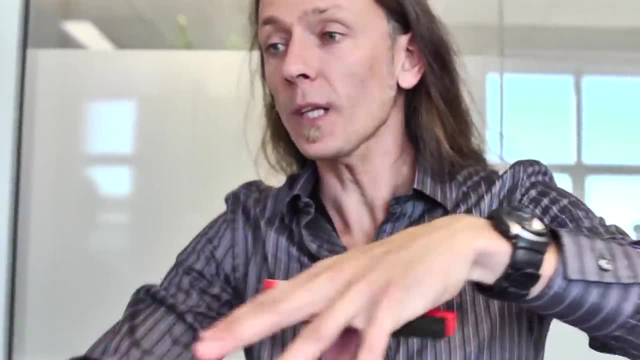 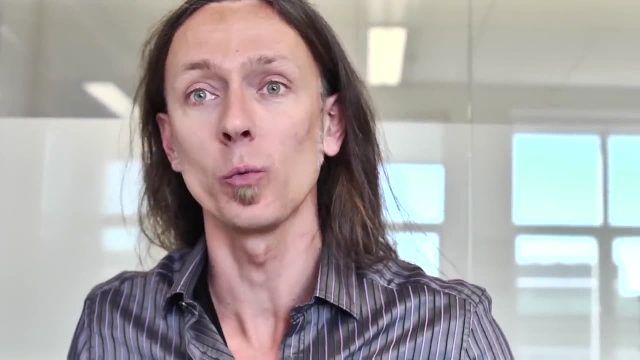 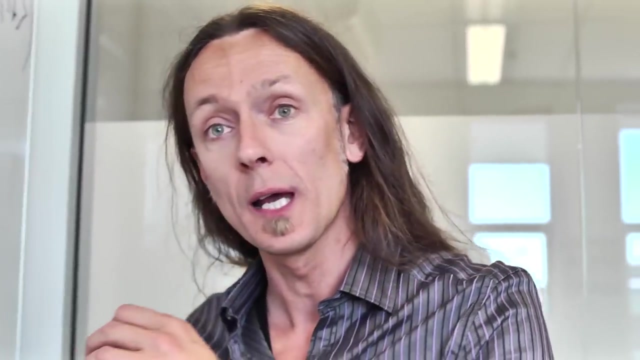 kind of computational parallelism. If you just want to watch a video in high definition or browse the internet or write some document in Word, they're not going to give you any particular improvement. if you need to use, They're not going to give you any particular improvement. if you need to use a classical, 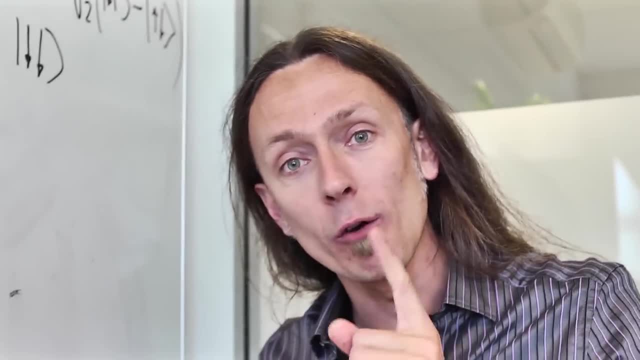 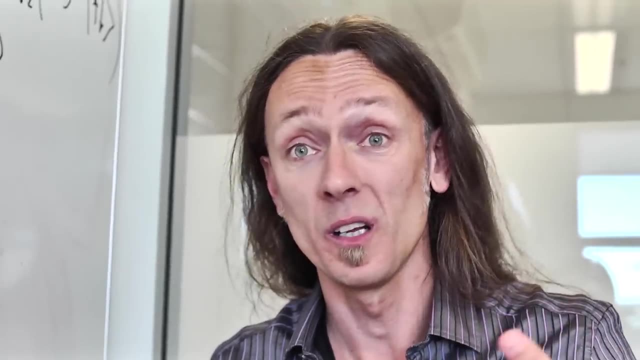 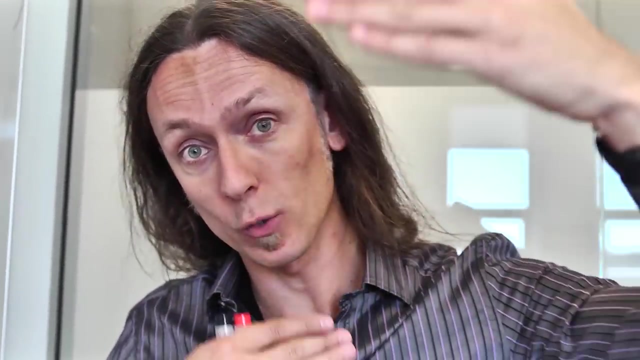 algorithm to get to the result. So you should not think of a quantum computer as something where every operation is faster. In fact every operation is probably going to be slower than in the computer you have on the desk. But it's a computer where the number of operations required to arrive at the result is exponentially.